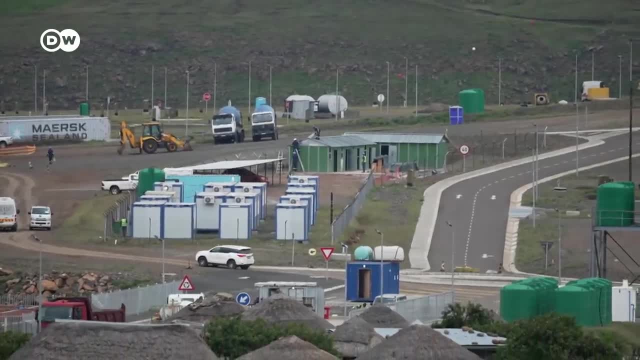 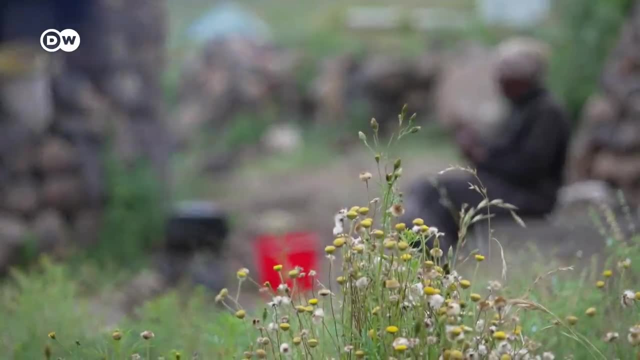 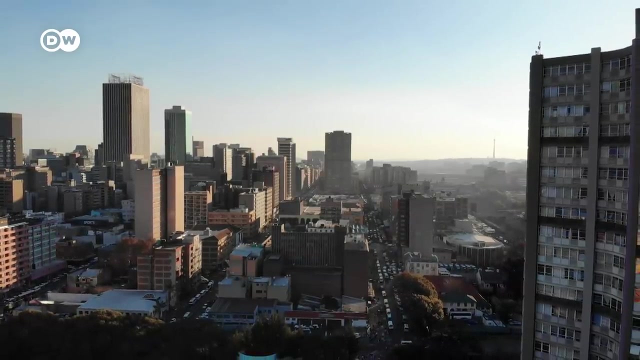 The cornfields and grazing land now house construction workers. Far from leading to greater prosperity, the dam has brought misery for residents, driving 8,000 people from their homes. The water will flow to South Africa's financial hub, Johannesburg, 400 kilometers away. 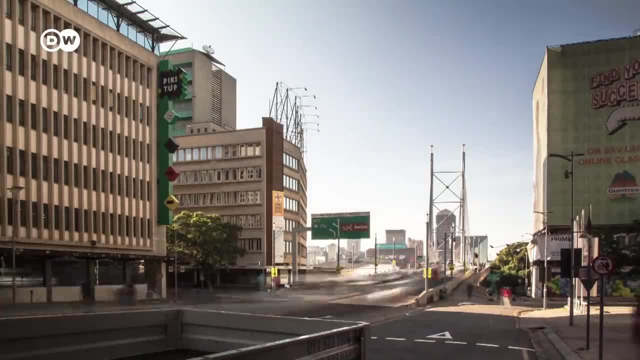 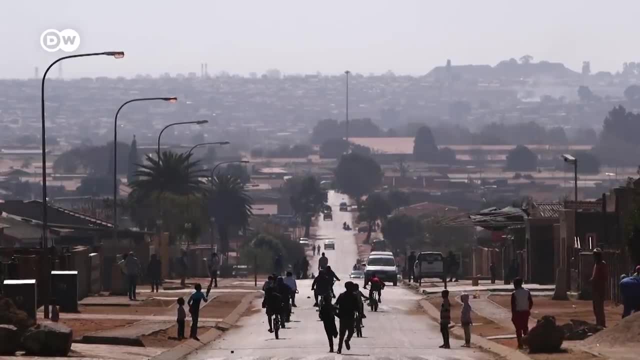 For the 16 million people in the city and surrounding province, Lesotho's dams are vital and already provide 60% of their water. Since the project is financed with South African taxpayers' money, Julius Kleinhans has been monitoring it for a long time. 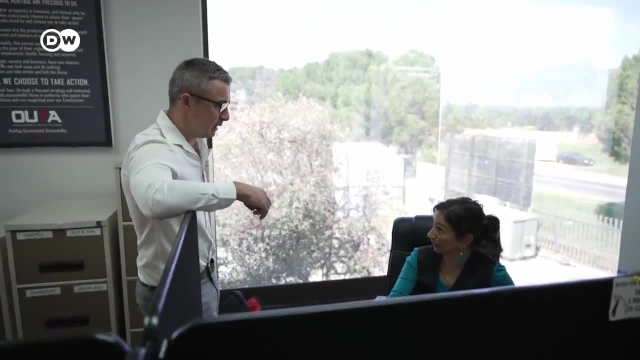 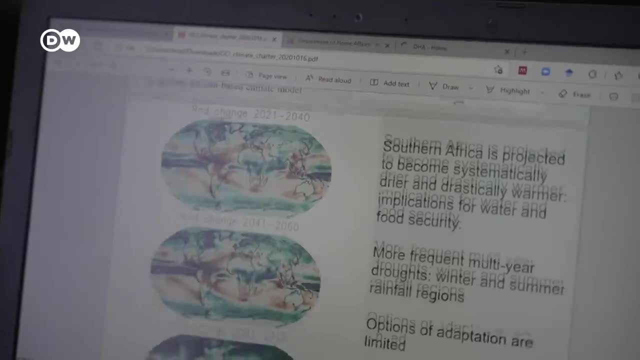 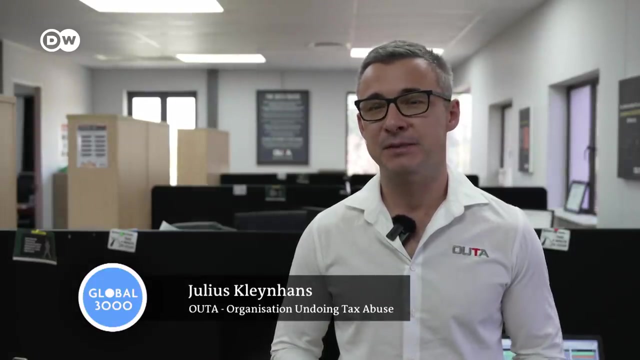 He works for the organization ALTA, which seeks to expose corruption and mismanagement. Urbanization is taking place and future development and expansion of business needs more water, And the problem is we're only very limited to the water that we have in South Africa. 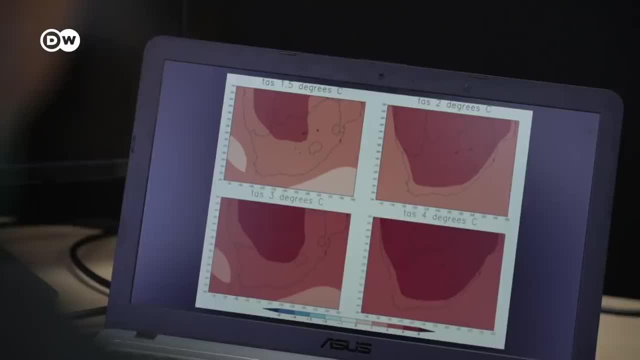 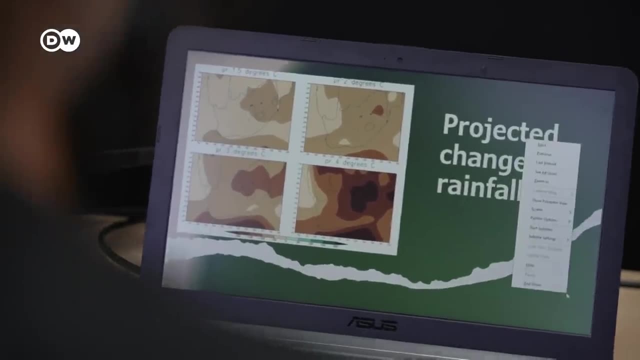 And the problem is we're only very limited to the water that we have in South Africa. And the problem is we're only very limited to the water that we have in South Africa. We don't have innovative technologies and circulated infrastructure yet to recycle water. 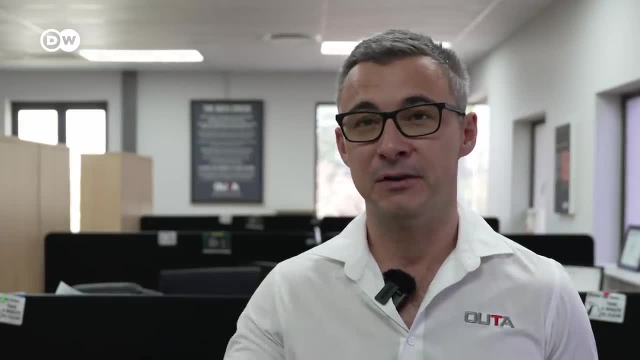 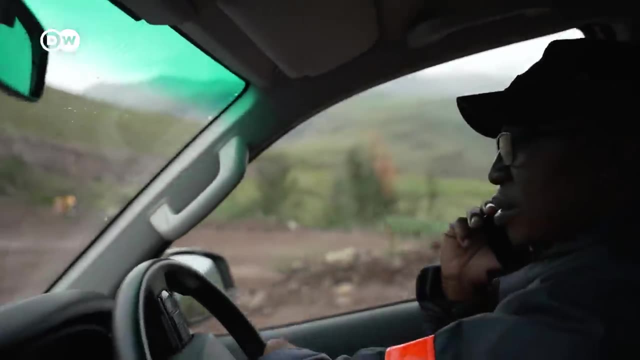 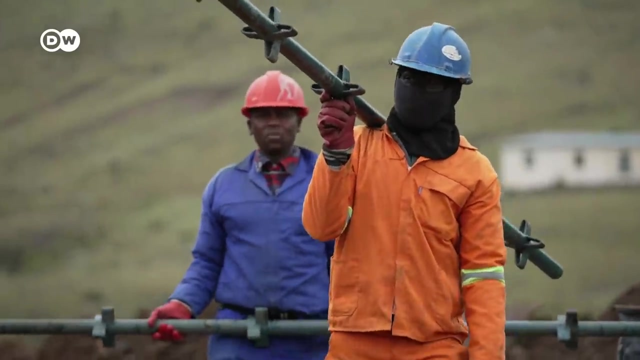 And currently we're highly relying on the Lesotho Islands Phase 2 scheme to provide future demands. It's one of the largest infrastructure projects in Africa and is supposed to benefit both sides. South Africa pays Lesotho nearly 70 million euros a year for the water. 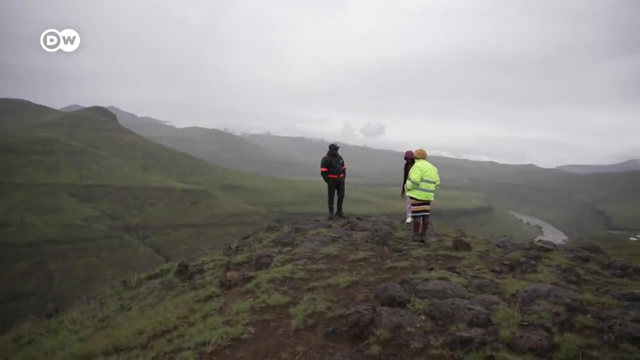 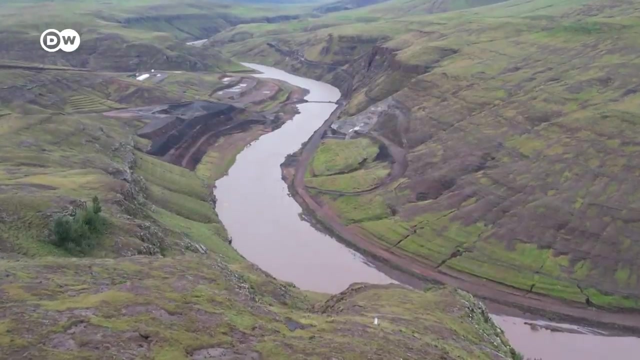 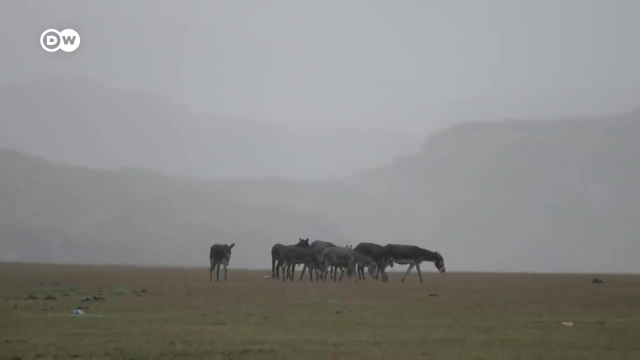 electricity for its population. The local project manager from the Lesotho Highlands Authority tells us that in five years time, the dam wall will stand right here. 5,000 hectares of land will then be flooded. As we are all aware, this kind of projects would have social impacts and 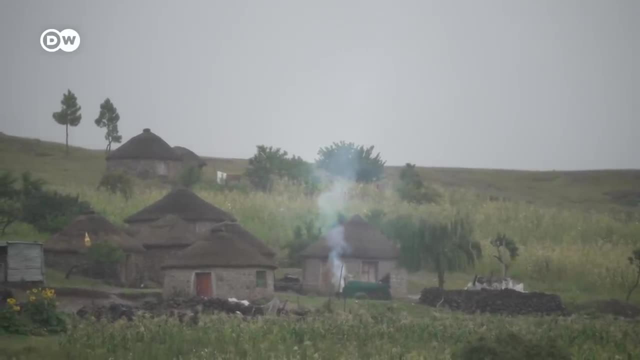 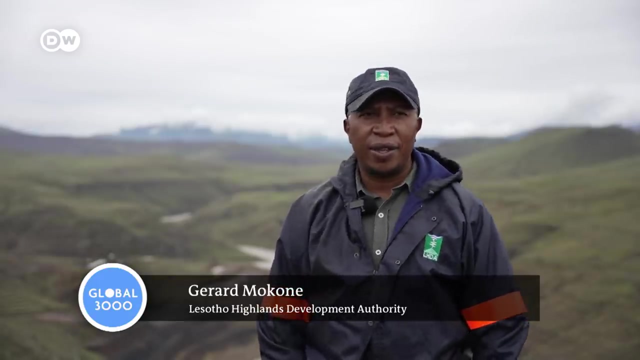 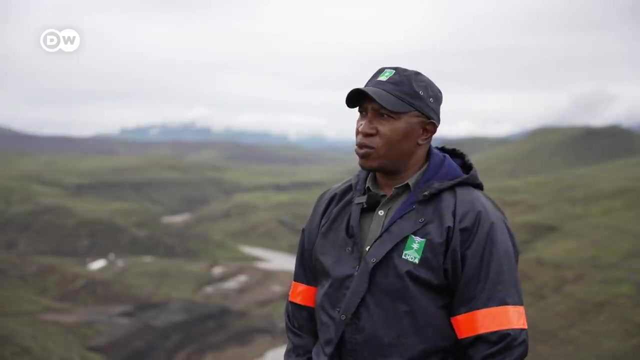 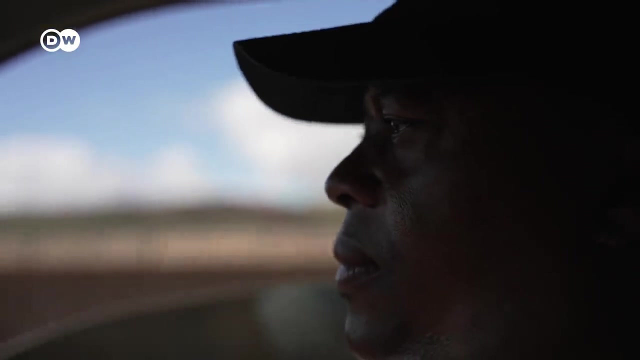 environmental impacts and we, as the project, have a number of programs which had been discussed and agreed with the communities as ways and means of mitigating against the loss of land and the loss of grazing areas and production land. Mutusi Sekwi heard exactly the same promises 24 years ago, when the 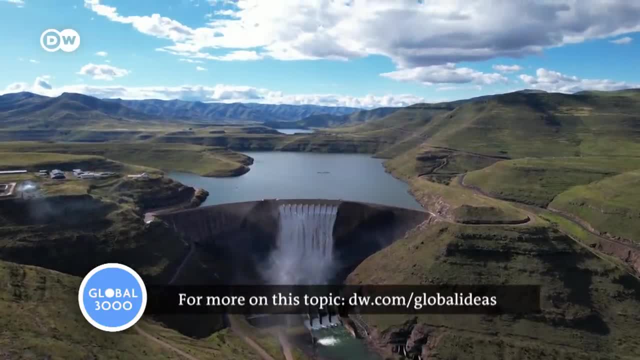 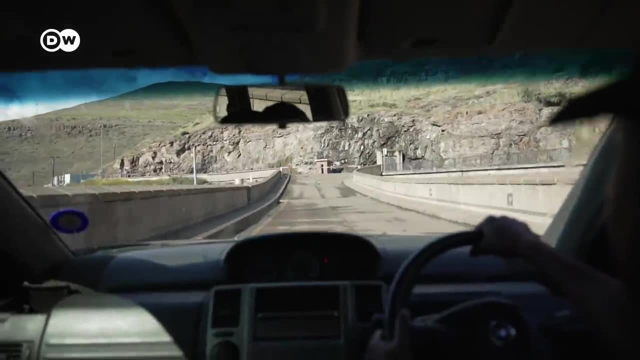 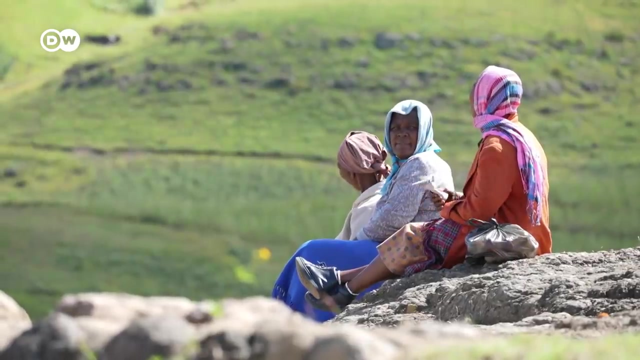 Katza dam was built. All other dams feed their water into this reservoir, from where it's piped to South Africa. Sekwi works for the Sayanoli legal center. It's helping local people like here in the village of Mapalang to now claim the compensation they were promised. 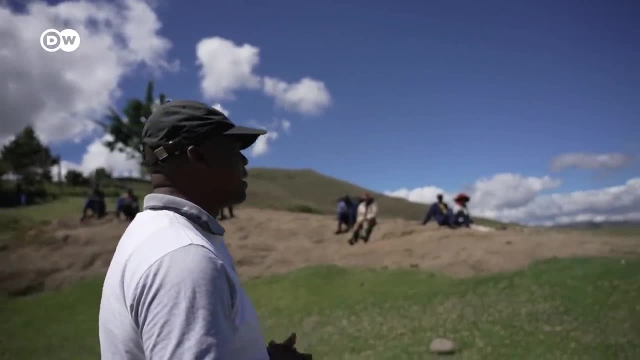 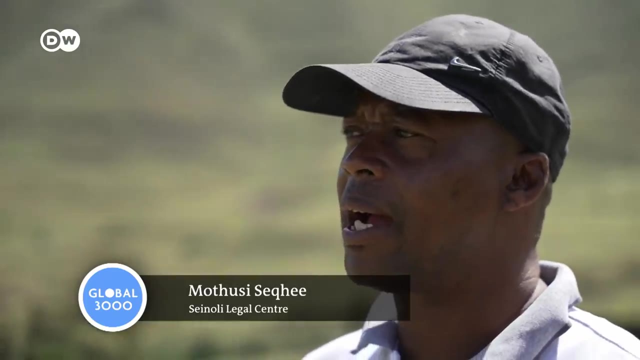 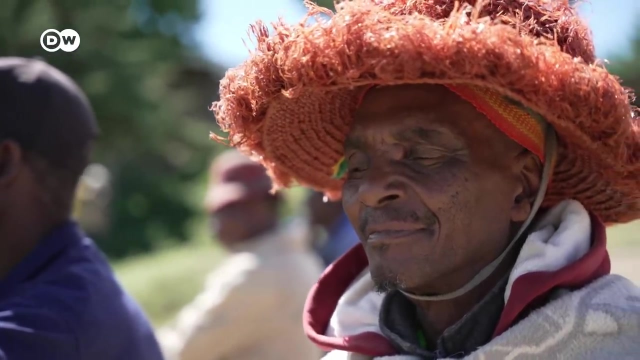 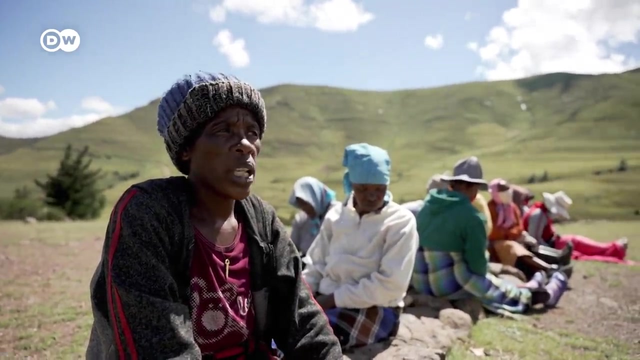 As everyone knows, you were severely impacted by the construction of the dam. Your rights have been trampled on and we all know why your water springs have run dry. We had decided to use the money to get our village connected up to electricity, but the Development Authority has done nothing. We're still waiting for power in. 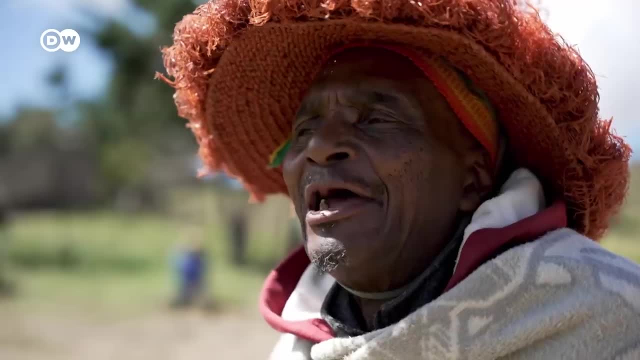 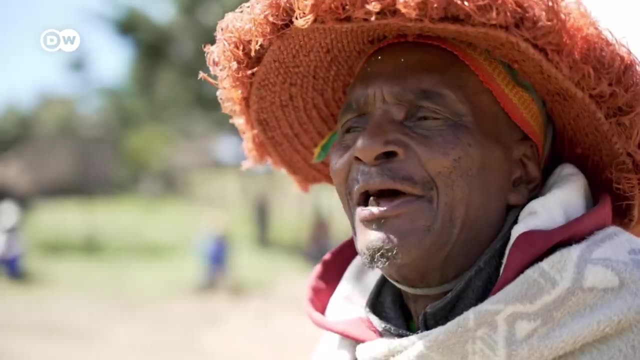 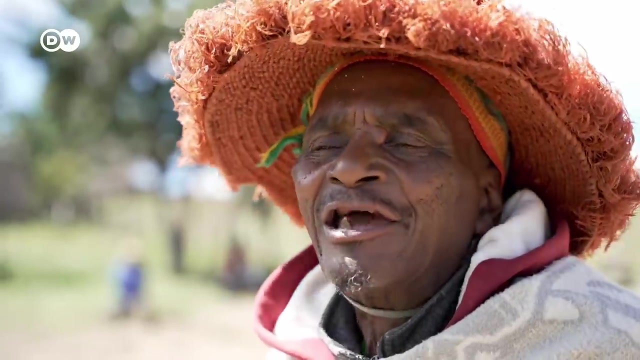 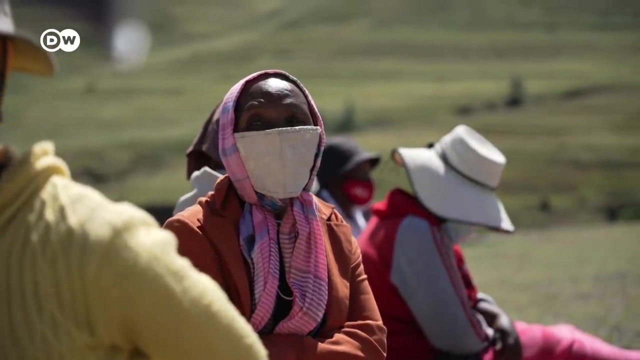 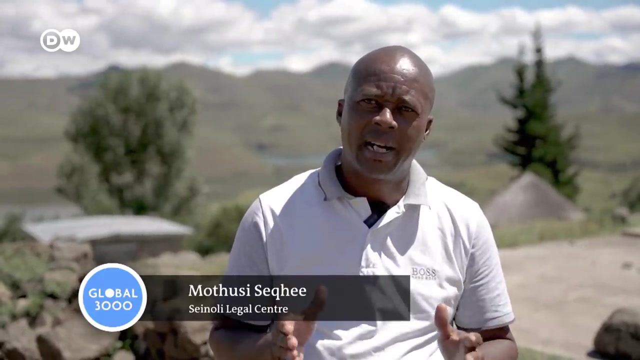 Mapalang. They also promised us compensation for the loss of our homeland and the pain we had because of the resettlement. Some people here got injured during the move, but to this day we have not received anything. The project was conceived by two undemocratic governments of 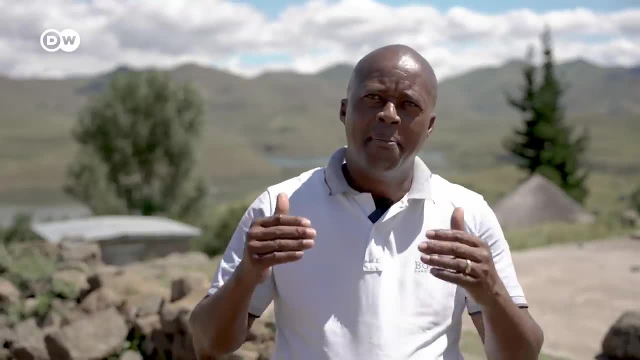 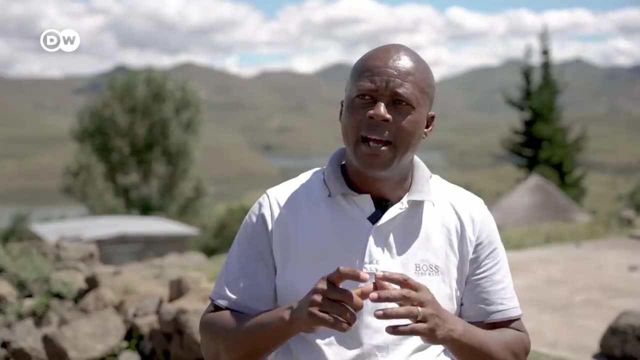 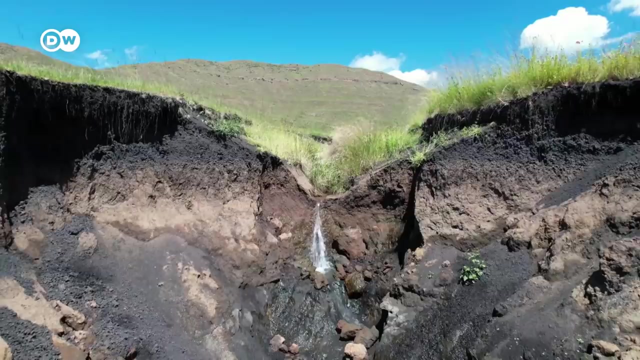 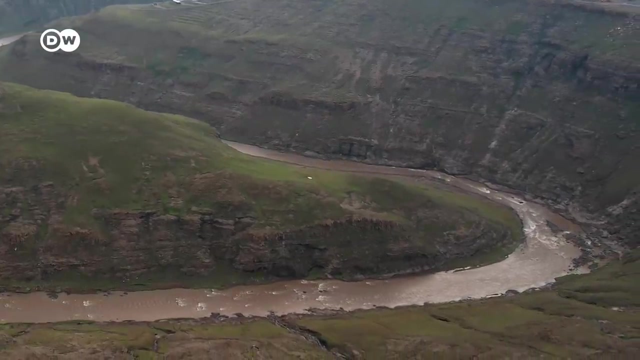 South Africa, The apartheid regime and the military regime in Lesotho Those governments had decided on did not have a mandate from the people. There is a need for the review of this treaty. The project is also threatened by massive soil erosion. The construction of the dams, 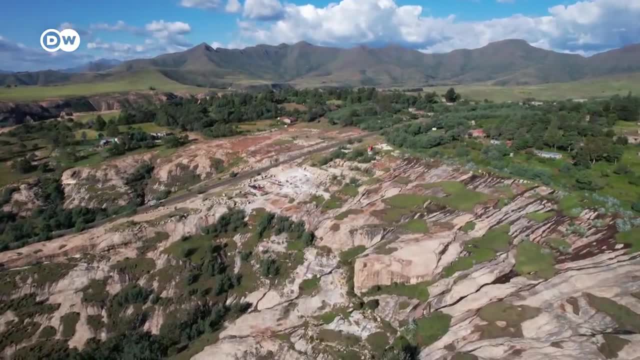 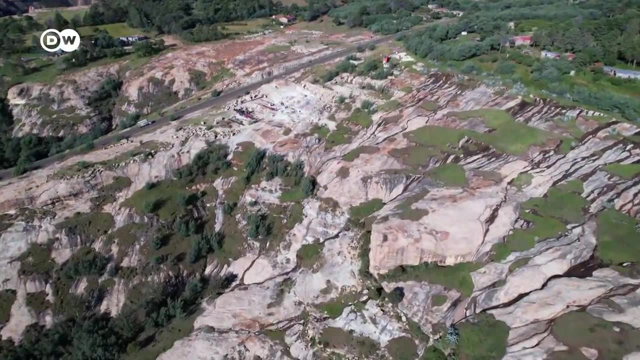 along with overgrazing and climate change, mean that more and more soil is being eroded by the rain and ends up in rivers as sediment. In many places, only bare rock remains. Taolo Tisseli is a consultant for a national project. 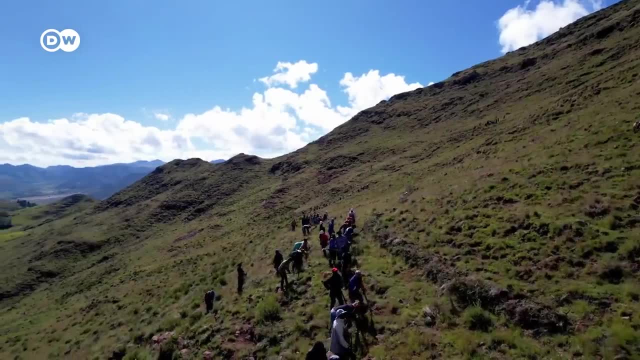 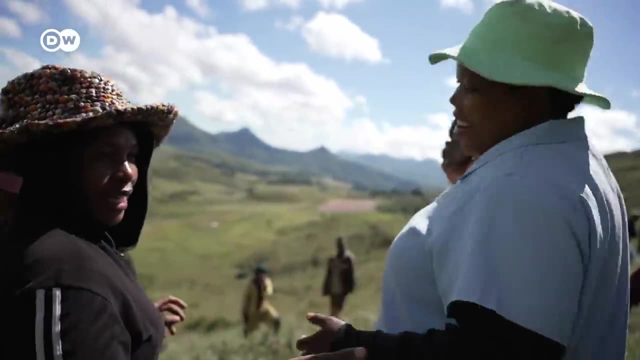 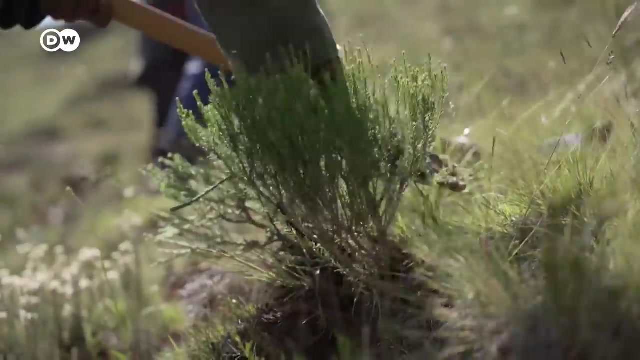 that aims to protect Lesotho's rivers. Workers here are building low walls into the hillside to reduce the speed and force of rainwater runoff and prevent erosion. They also remove invasive shrubs that would otherwise wipe out endemic plants whose roots help to keep the soil in place.